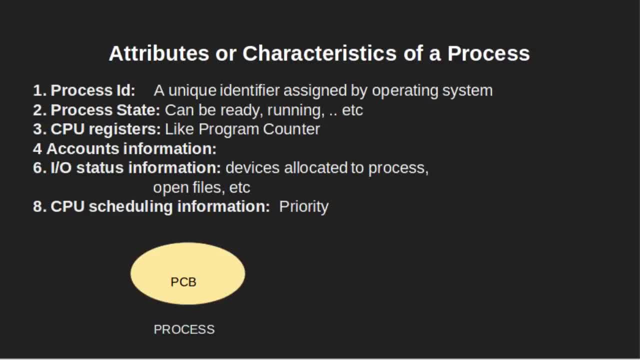 Attributes or characteristics of a process. First is process. First is process ID, A unique identifier assigned by the operating system to each process. Second is process state. This can be ready, running, waiting, etc. CPU registers are like program counters. 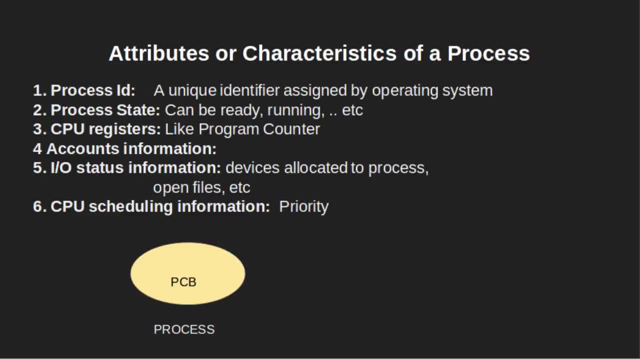 Fourth is the account information. Fifth is input output status information, For example devices allocated to a process, open files, etc. CPU scheduling algorithm, For example priority: Different processes may have different priorities. For example, a short process may be assigned a low priority. 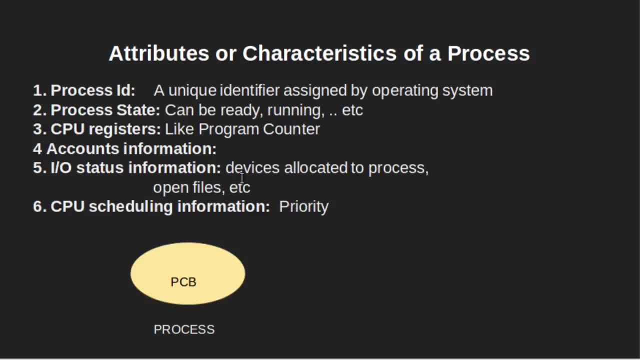 In the shortest job first schedule. All the above attributes of a process are also known as context of the process. Every process has its own program control block. That is, each process will have a unique process control block. All the above attributes are part of the process control block. 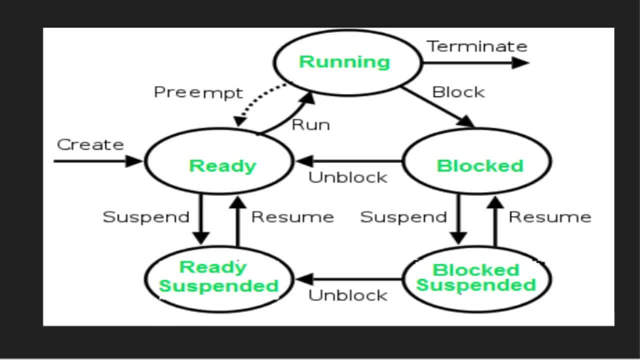 States of a process. Initially, process will be in new state. It means process is under creation or a process is being created. Once the process is created, it will be in new state. Once the process is created, it will be moved to the ready state. 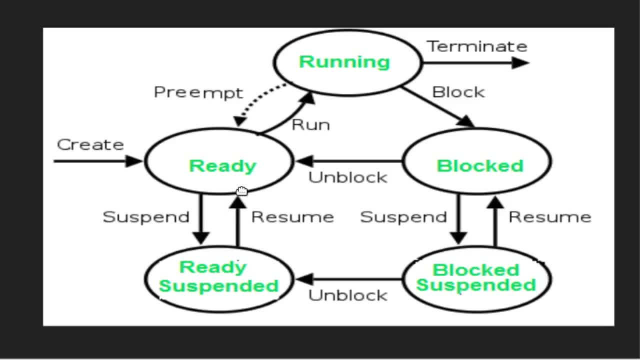 In the ready state. there will be multiple number of processes. One of the process will be selected from the ready state and dispatched onto the running state. In the running state, process occupies the CPU and executes the instructions of the process In the running state. 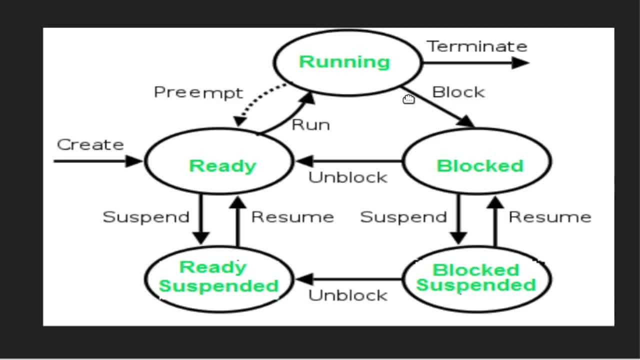 one process can be, at any point of the time, Wait or block state. If the running process required any input output, then it will come to wait state. In wait state there will be multiple number of processes. It means multiple process will perform input output operations simultaneously. 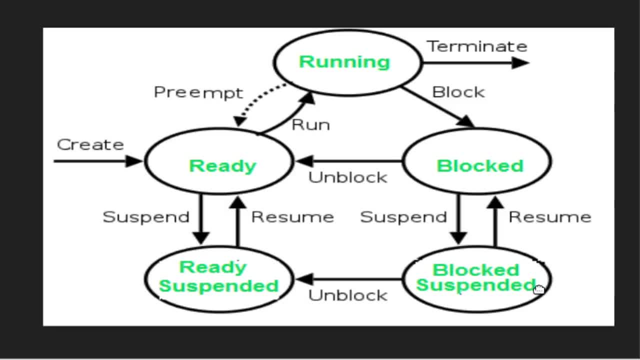 Blocked, suspended. If the resources are not sufficient to maintain the process in the wait or block state, then some of the process, with low priority maybe, will be suspended and they will be moved to the suspended block state. In this the process reside in the backing store. 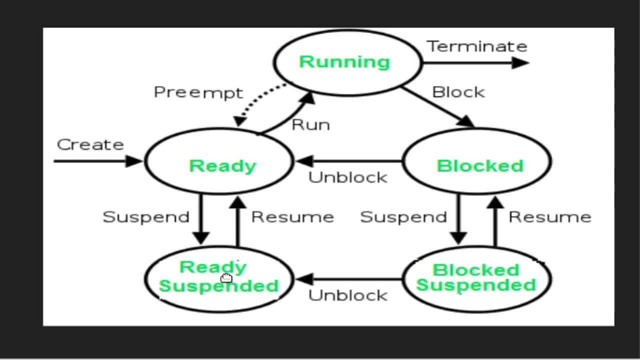 Ready- suspended. If the resources are not sufficient to maintain the process in the ready state, then some of the processes will be suspended and moved to the very suspended state. Here also, process resides in the backing store that is secondary storage. Terminated or completed state. 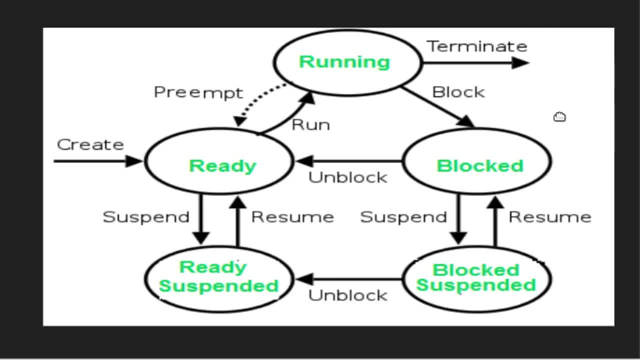 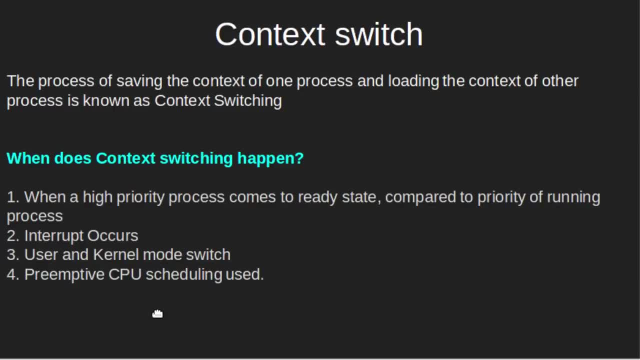 When the process completes its execution, it is moved to terminated state. Context switch- The process of saving the context of one process and loading the context of another process is known as context switching. So when does context switching happen? When a high priority process comes to ready queue. 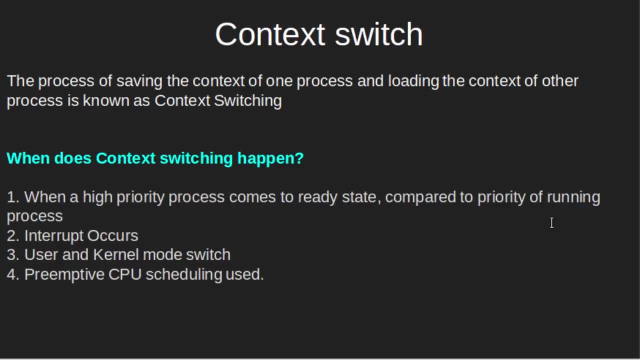 compared to priority of running process. So definitely higher priority will be given, more priority and low priority process will be stopped and high priority process will start Any interrupt occurs. If any interrupt occurs, it has to be handled at that time. User and kernel mode switch. 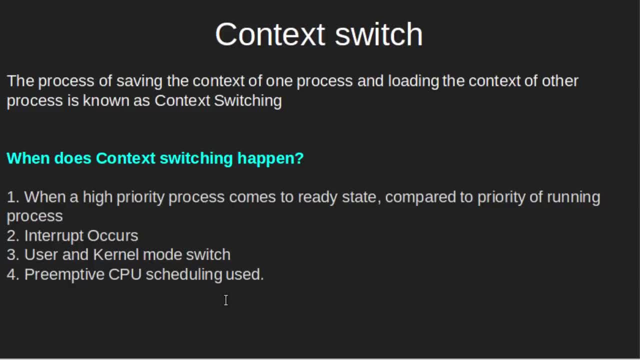 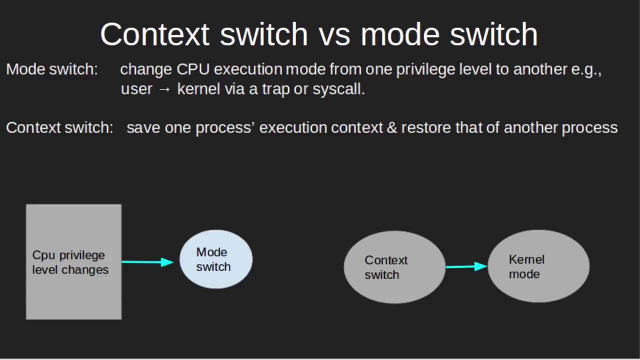 Whenever there is a need of kernel mode, it has to be switched urgently. So there also context switching will happen. Preemptive CPU scheduling used Context switch versus mode switch. A mode switch occurs when CPU privilege level is changed, For example. 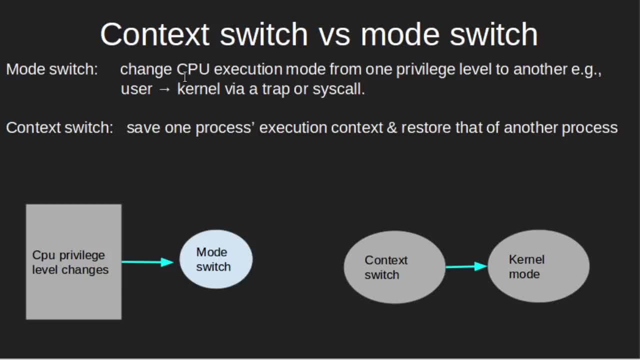 when a system call is made or a fault occurs, The kernel works in more privileged mode than a standard user task. If a user wants to access things which are only accessible to the kernel, a mode switch must occur. The currently executing process need not to be changed during a mode switch.